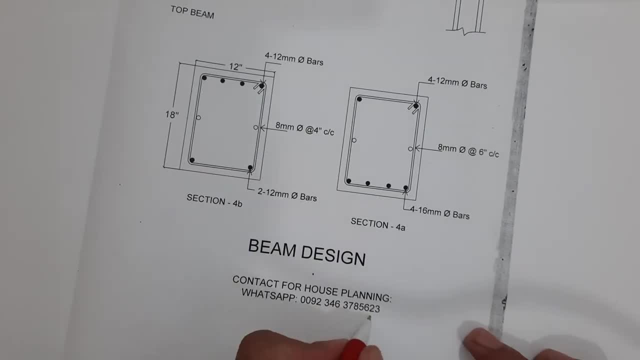 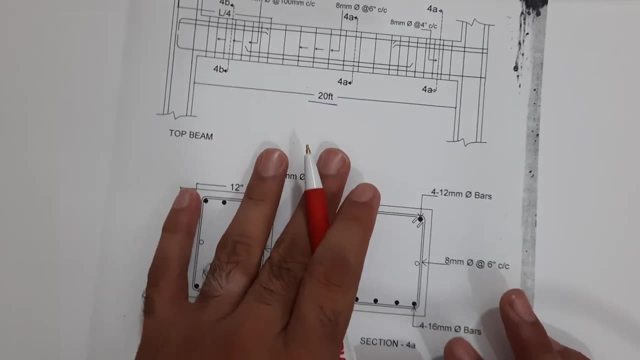 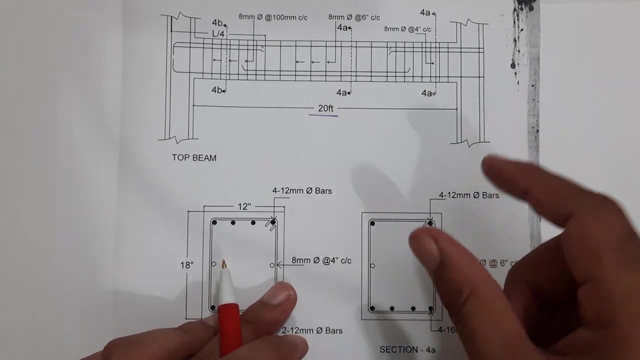 structural drawing 3D animation for any type of building. so you can contact me on this WhatsApp number. This is paid services, not for free. The size of beam for 20 feet span you can keep. this is specially for up to three-story building G plus two ground floor. 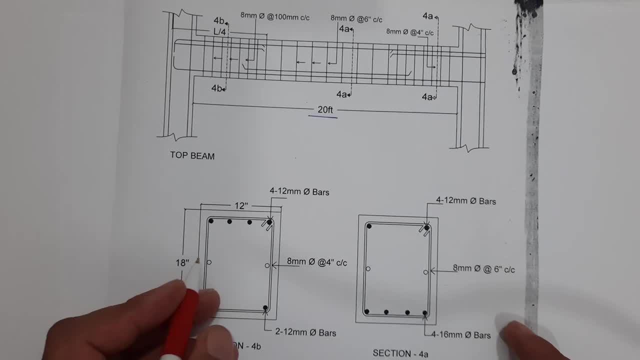 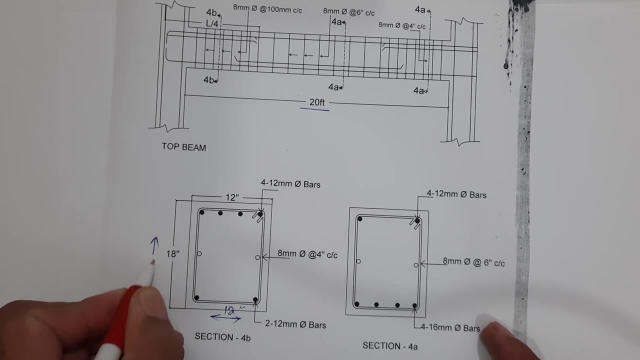 first floor and second floor. Here, guys, you can see, the size is 12 by 18 inches. Width is here 12 inches and depth is here 18 inches. So this is its depth, okay, and this is width, So 12 by 18. 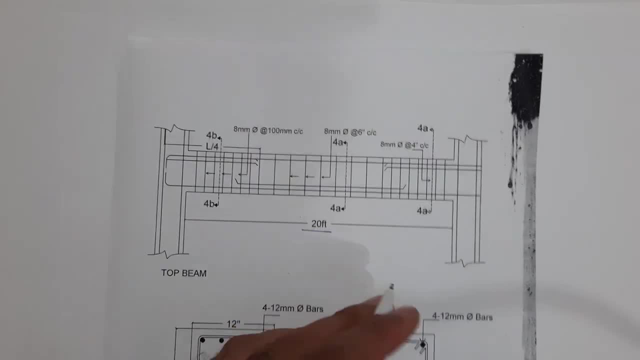 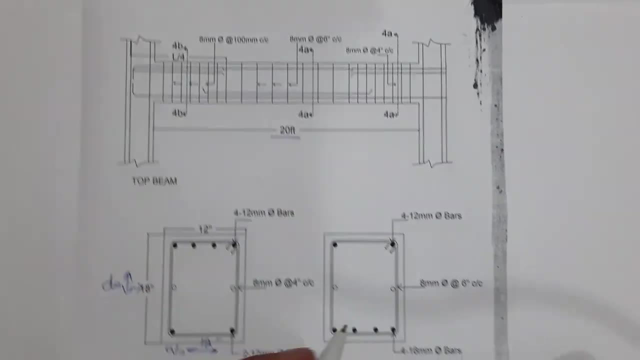 inches you can keep the size of beam. Here, guys, you can see, this is the long section of beam and this is the cross section of beam. We have two sections. That's why, specially for its steel reinforcement, This is section 4A. Here, guys, you can see, this is. 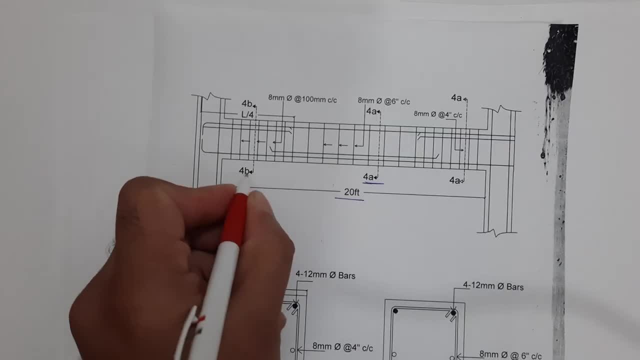 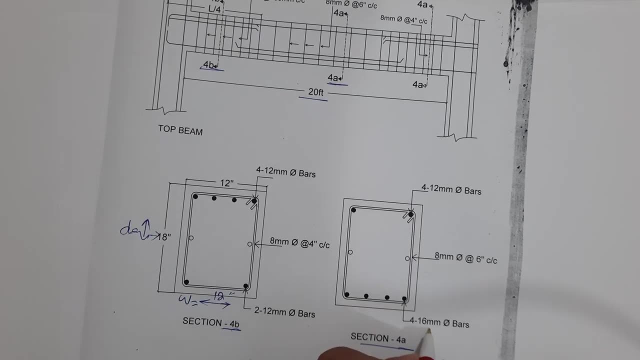 section 4A, and this is section 4B where you can see the section 4B. In section 4A, as you can see, guys, we have four steel rods at the bottom. dia is 16 millimeter, Four numbers at the bottom. 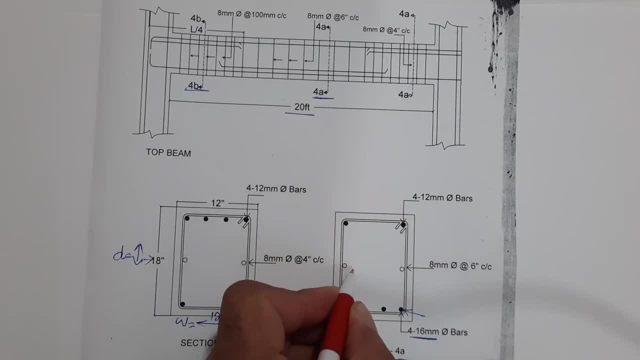 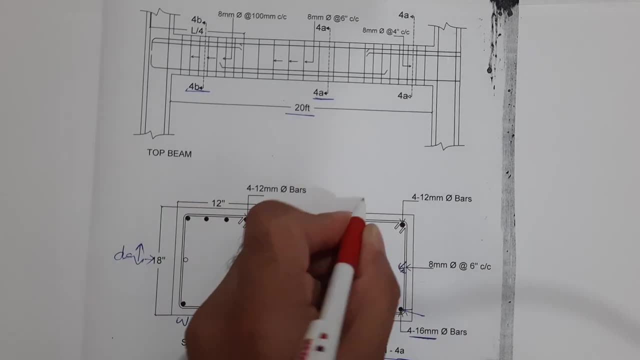 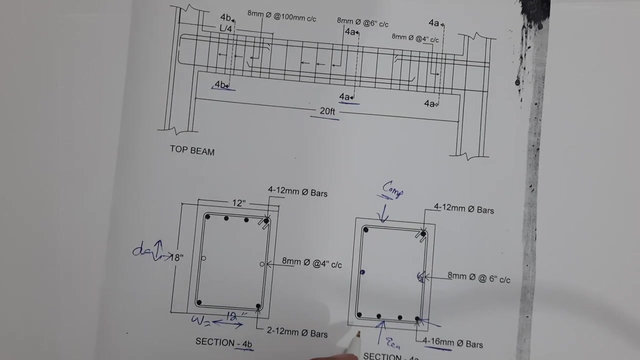 dia is 16 millimeter and two numbers, four numbers in upper portion, Two at the middle. guys, you can see these are sidebars and two are upper portion steel reinforcement. Or you can say: this is compression zone, okay, And this is tension zone. So therefore, guys, 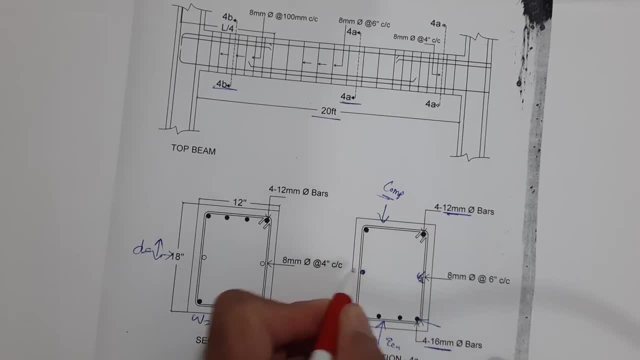 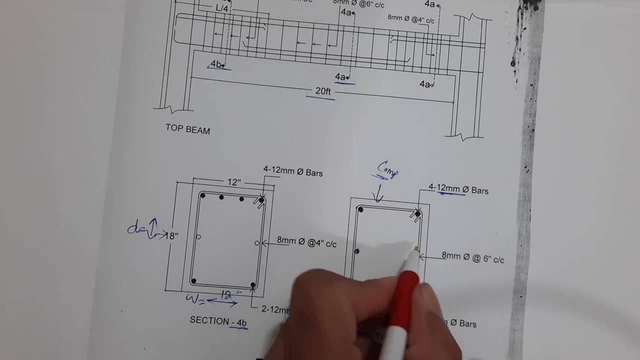 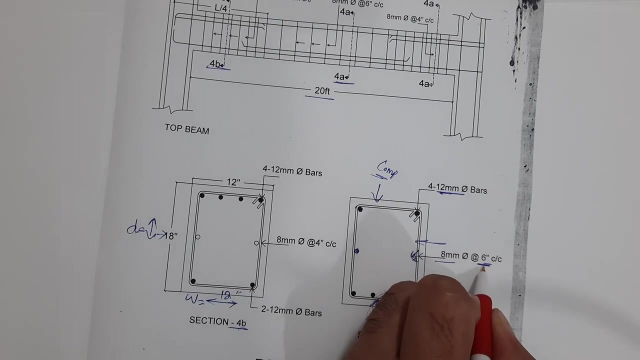 the dia is 12 millimeter. So these four steel rods dia is 12 millimeter and bottom tension zone steel reinforcement bars are 16 millimeter, If you see, guys, the stirrup, so the stirrup dia is 8 millimeter with the spacing of 6 inches. Okay, this is the spacing of 6 inches center. 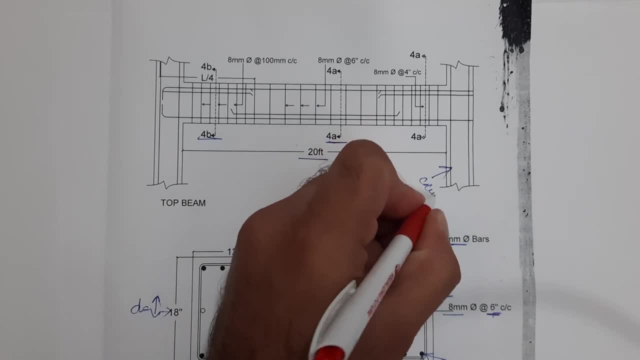 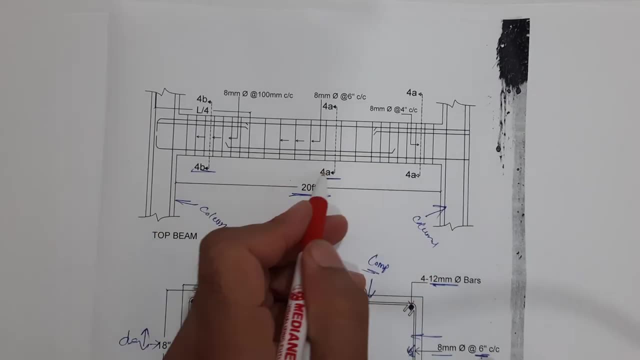 to center. Guys, you can see, this is column and this is other column. It means these are supports and the span is up to 20 feet. Here, guys, you can see in section 4A we have four bars at the bottom and two at top portion. But if you 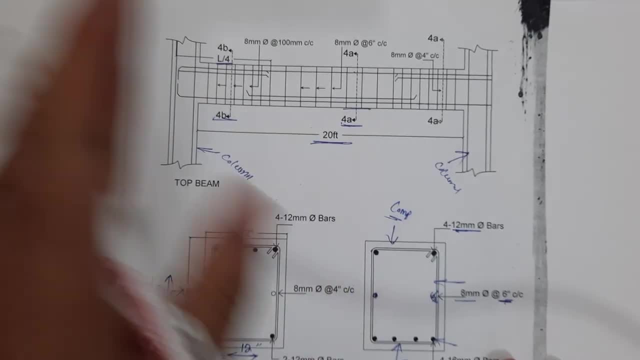 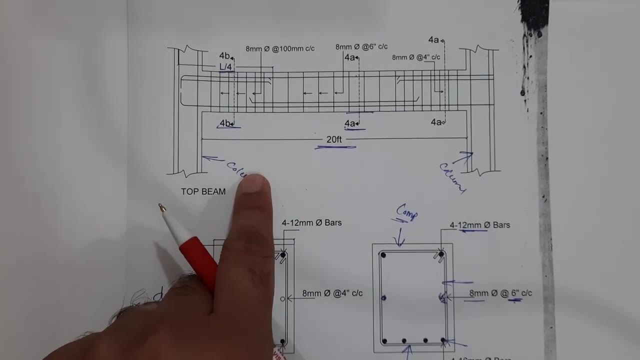 see, guys, this is L by 4 distance Where we have negative bending moment. as I told you in many videos, to resist negative bending moment, we are providing extra steel rods or bent up bar. But here, guys, we don't have the bent up bar, because bent up bars are same, like this: 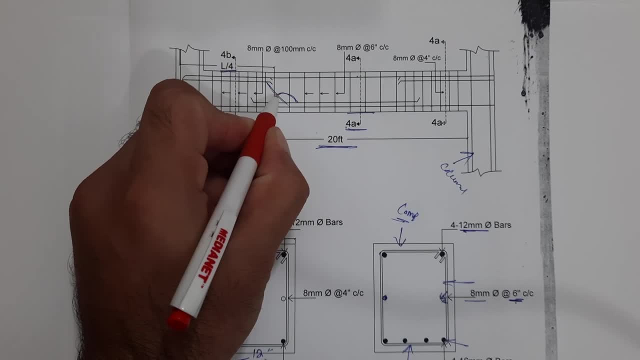 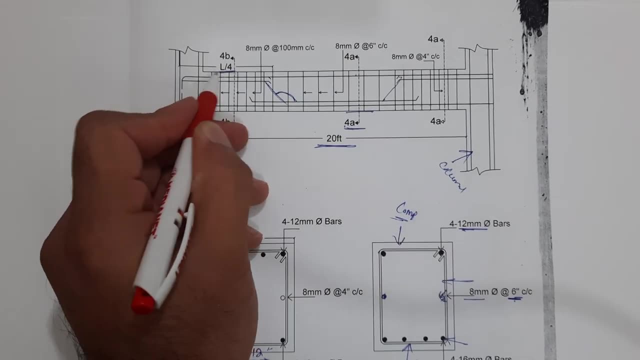 We are making the angle here from 45, to 60 degree. Also same here, But this is not crank bar or bent up bar, But here we have extra steel rods at the distance of L by 4. L by 4 means 20 feet divided by 4, where we have 5 feet. So at 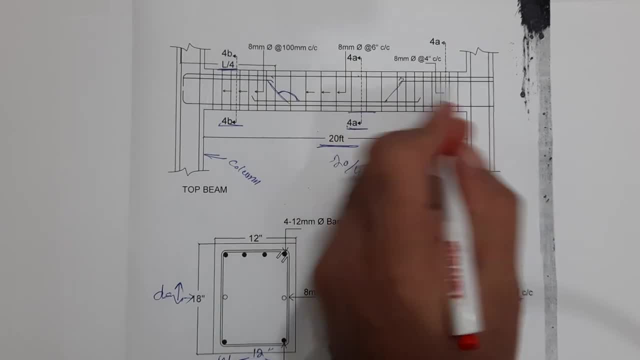 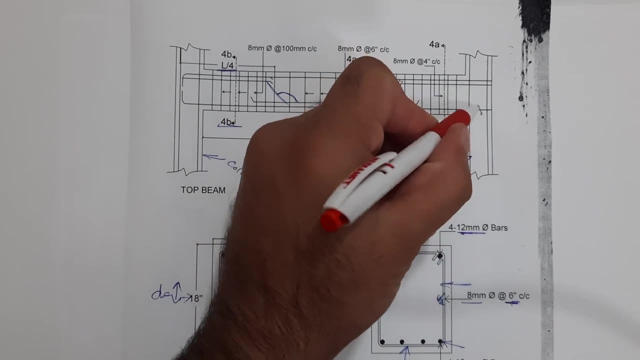 the distance of 5 feet. we have extra steel rods, also left and right side, because we have the support. So near its support, we have negative bending moment. Let me make a diagram for this. So, guys, here you can see this is negative bending moment. at the middle we have positive bending. 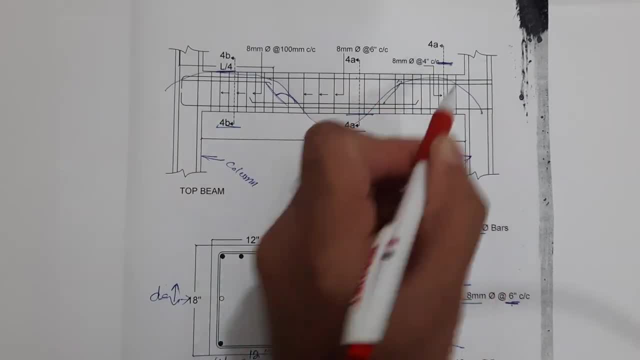 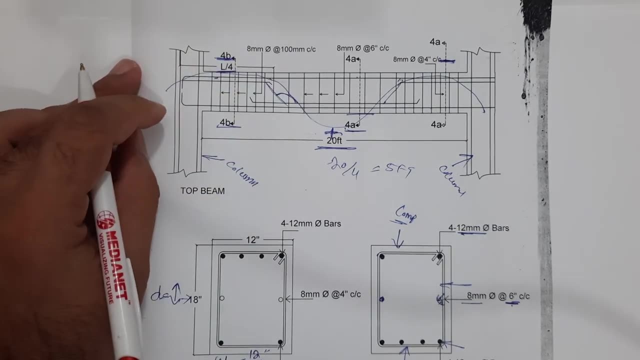 moment. Again we have negative bending moment moment. so here we have negative bending moment, here where we have l by four distance, and here we have positive bending moment. to resist negative bending moment, we are providing extra steel rods, okay. so therefore, guys, you can see at the section of 4a we have four steel rods. 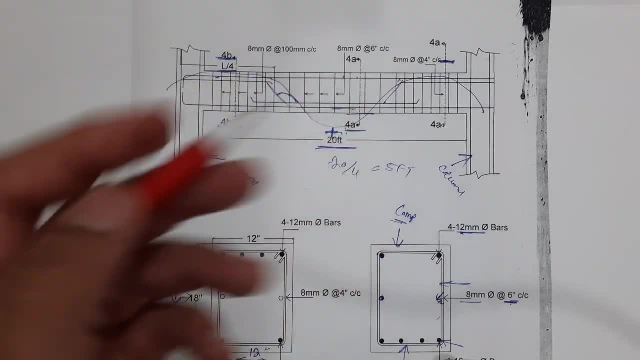 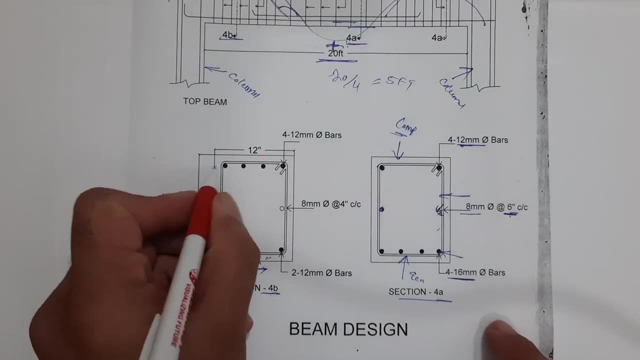 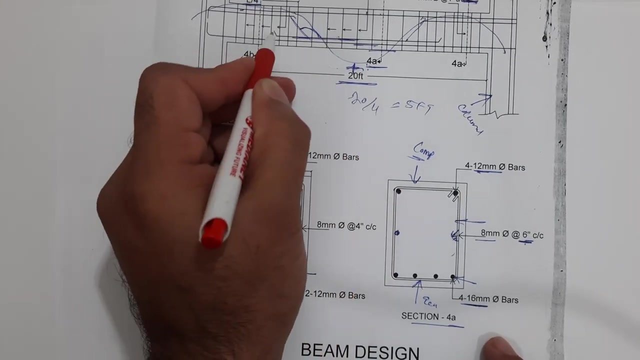 at this section to an upper portion, okay, and to our sidebars, if you see the section b 4b at the distance of l by four specially we did this okay, so we have here two steel rods at the bottom, guys, you can see, because this is just to the distance of, so here you can't see at the distance of l by. 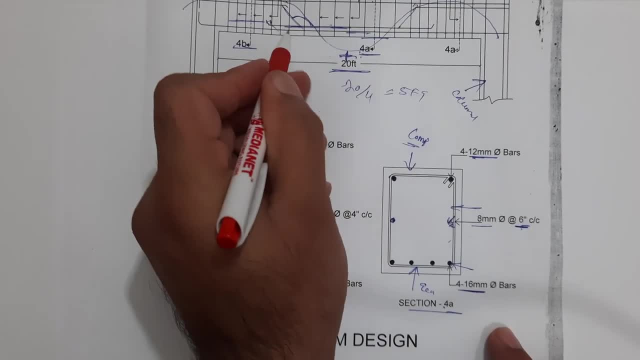 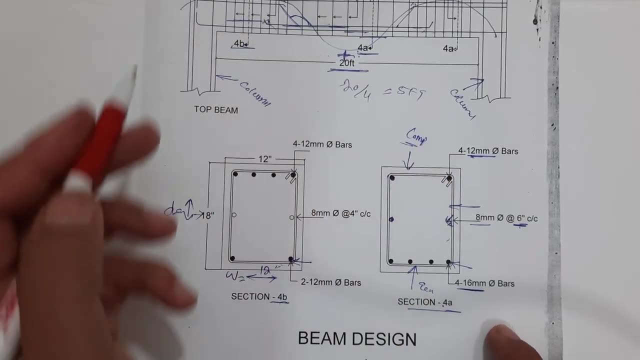 four- this is just at the distance of after l- by four. okay, from this side and also from this side. so therefore, we don't have this steel rods, this one. okay, as you can see the hook here we don't have. so therefore, in bottom portion, we have two steel rods in the corner. okay, which dia is here? 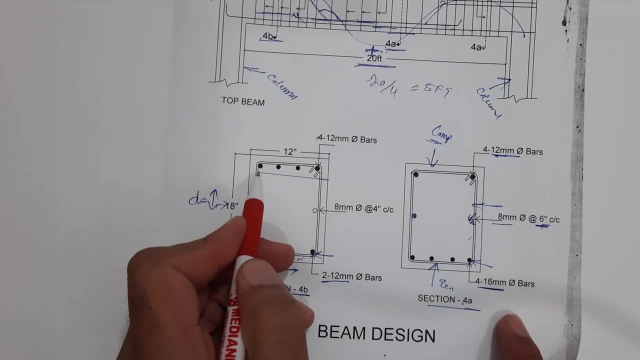 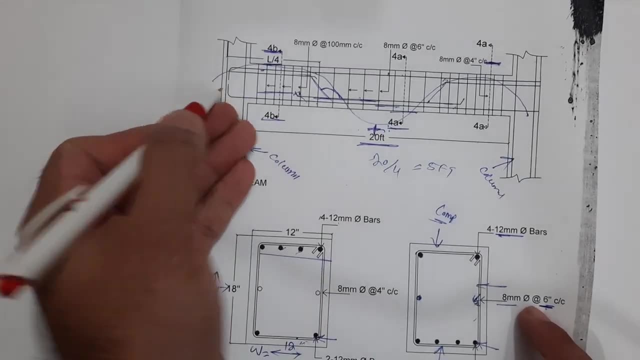 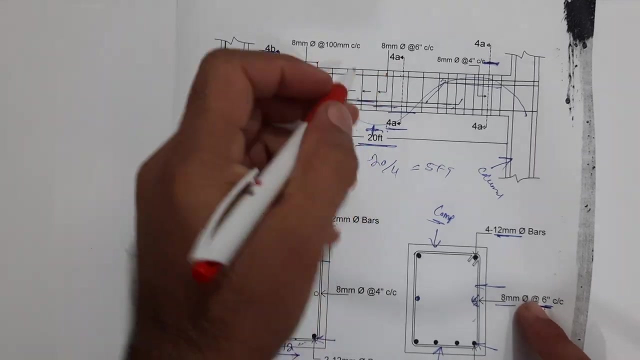 two numbers 12 millimeter and four numbers 12 millimeter in upper portion. okay, so therefore, guys, we have two extra steel rods here, you at the middle, to resist negative bending moment. here, at the distance of l, by four, we have same situation you can see at this side. so, guys, this is the topic for today, so next let me guide. 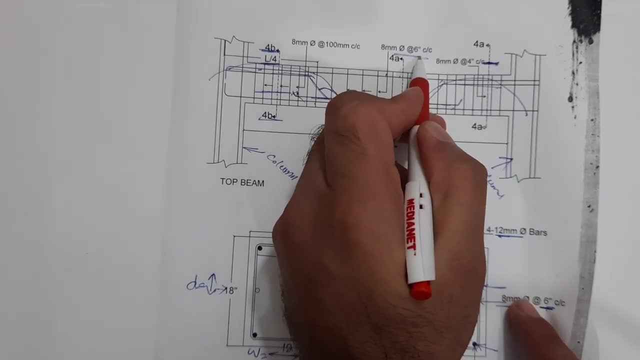 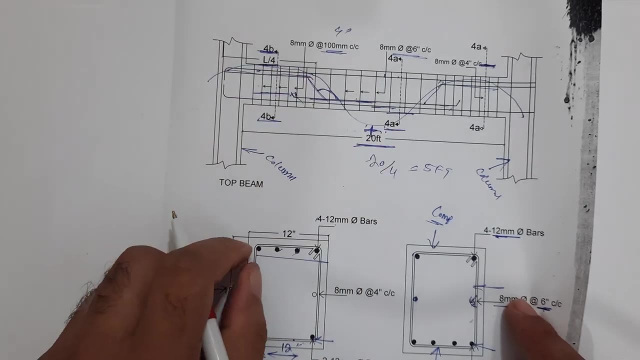 you for it stir up, so you can see the stir up spacing is here six inches, because we have positive bending moment, here we have negative bending moment. so therefore we have 100 millimeter or four inches center to center distance are spacing between the stirrups. okay, eight millimeter dia.